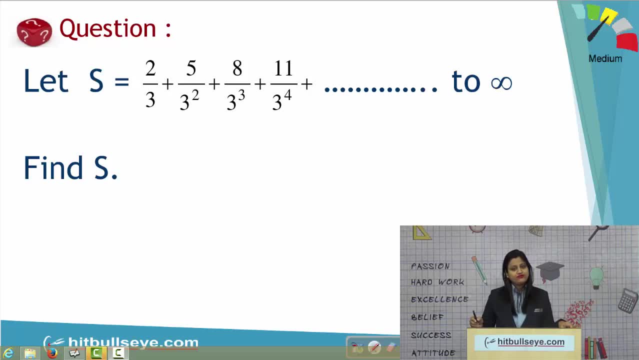 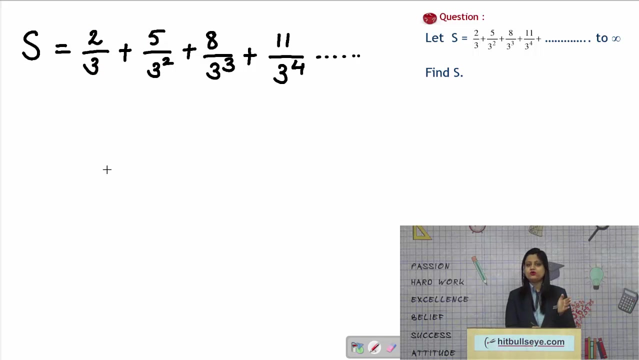 We want to calculate s. We want to find the sum of infinitely many terms. As you can see in the numerator, we have an arithmetic progression. What is the first term here? That is 2. What is the common difference? That is 3. And in the denominator, we have a geometric progression. What is the first term of this GP? 1 by 3. And what is the common ratio? That is 1 by 3 again. This is our first term and this is the common ratio of the GP. So, that is a combination of arithmetic progression and geometric progression. So, we call them AGP series, Arithmetico-Geometric Progression. We have a particular method to solve these kind of sums. Let us see the method. Then we will come to the shortcut. First of all, we will write a new formula which is 2 by 3 S Y times 1 by 3 S equals by common ratio, which is 1 by 3 in this case. So, it will become 1 by 3 S. Now, what will be the first term in this case? It will be 2 by 3 square. We will leave the first place empty. We will write the first term here, then take the subtraction. It will become 2 by 3 S, first term as it is. Now, 5 by 2 is equal to half. So, I have learned that two times half is equal to half. Now, you can calculate the first term. Let us check that. It is approximately 3 s divided by 1. Let us see. 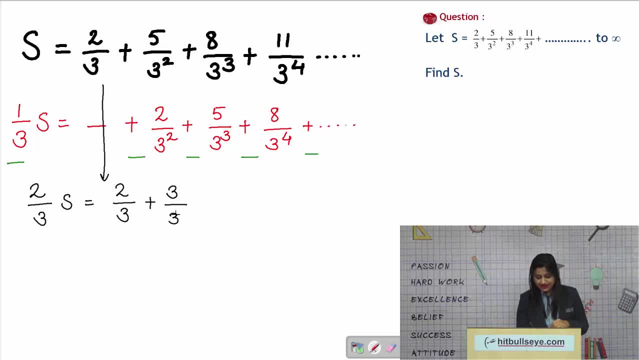 Now 5 minus 2, 3 since we have same denominator. Now you can see that second term onwards we have a pure GP, pure geometric progression and there are infinitely many terms in that GP. We have a formula to calculate sum of infinitely many terms of a GP. What is the formula? That is a upon 1 minus r where a stands for first term and r stands for common ratio. So we can write 2 by 3 s is equal to first term again as it is 2 by 3 plus. Now we will apply the formula. 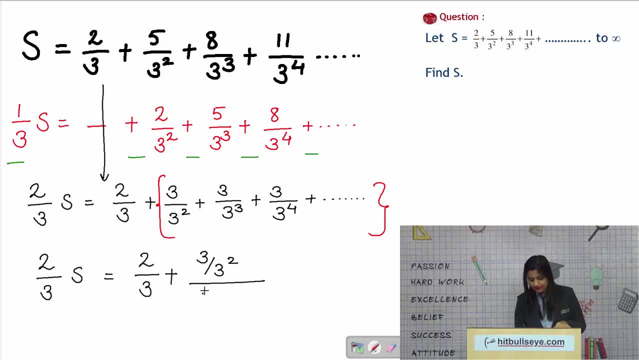 So it will become 3 by 3 square that is a upon 1 minus r which is 1 by 3 in this case. 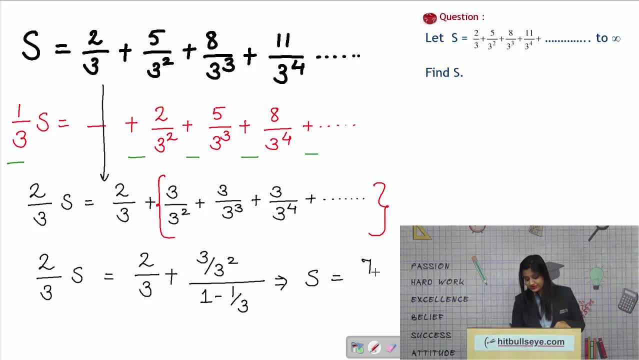 If you solve it you will get s is equal to 7 by 4. I am leaving the calculation part for you. 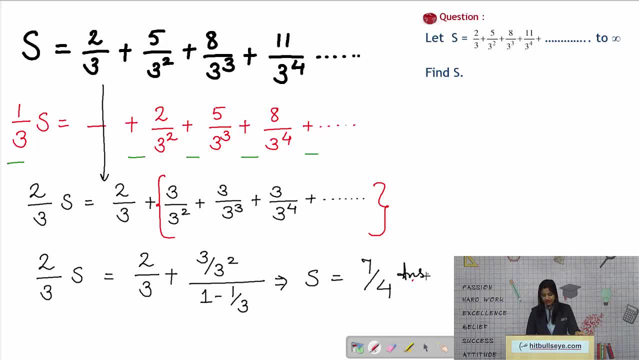 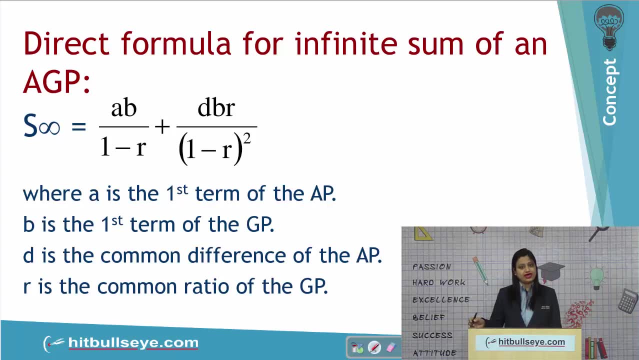 So this is the answer in this. 7 by 4. Now come to the shortcut. This is direct formula for infinite sum of an a GP. It says s infinity I mean sum of infinitely many terms. This is equal to a b upon 1 minus r plus d b r upon 1 minus r whole square where a is the first term of the a b, b is the first term of the g p, d is the common difference of the a p, and r is the common ratio of the g p. Let us apply the shortcut. 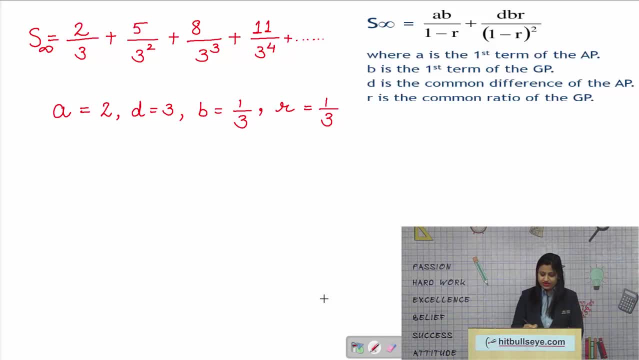 I am taking the previous sum only. So if we apply this formula, s infinity will become a into b divided by 1 minus r plus d b r upon 1 minus, whole square so if you solve it you will get the same answer which comes out to 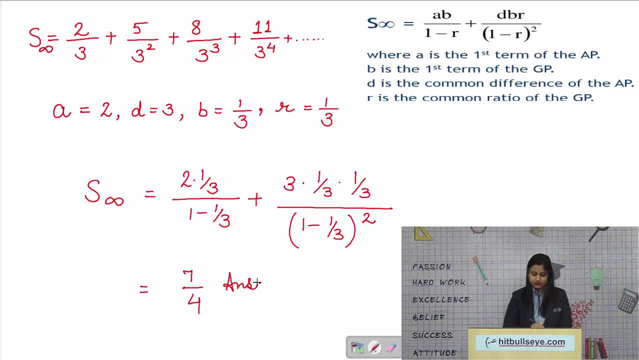 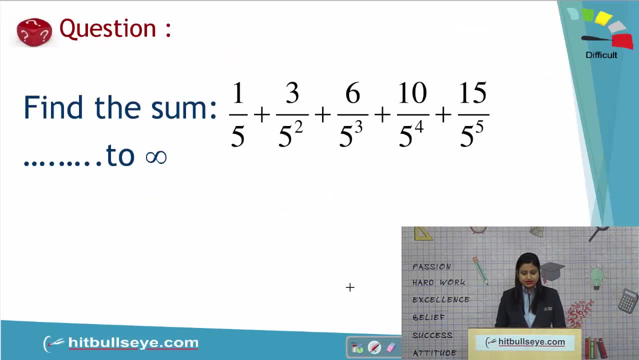 be 7 by 4 now let us move further there is one more question based on AGP series again we want to find the sum 1 by 5 plus 3 by 5 square plus 6 by 5 cube plus 10 upon 5 raised to power 4 plus 15 upon 5 raised to power 5 and so on up to infinity in the numerator if we take the difference here the difference is 2 then 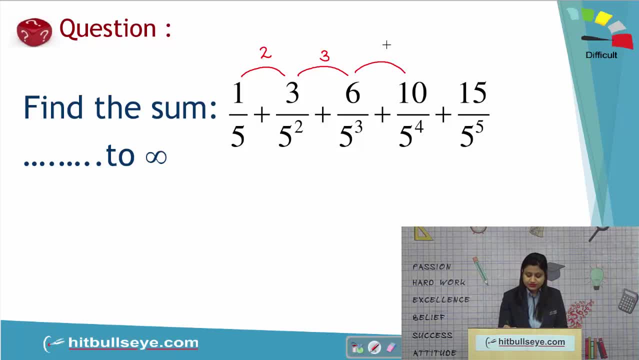 we have a difference of 3 not the same difference 4 5 so that is not a direct question of AGP so we cannot apply the direct form 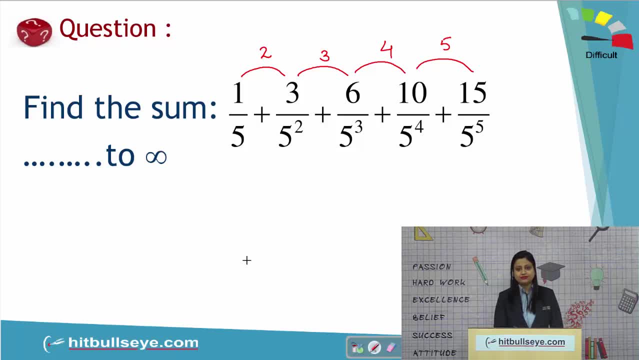 equation so we cannot apply the direct form formula for finding the infinitely many terms sum of AGP but in the second step 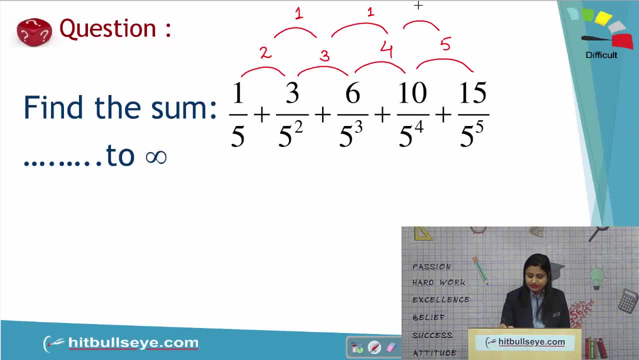 if we see it becomes an AP arithmetic progression so how can we solve these 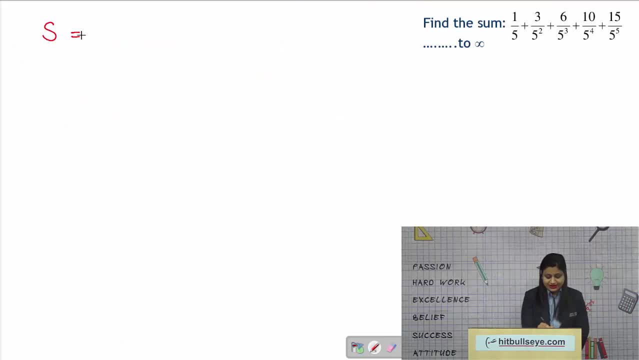 kind of sums we'll apply the same technique let s is equal to 1 by 5 plus 3 by 5 square plus 6 by 5 cube plus 10 by 5 raised to power 4 and so on up to infinity what is the common ratio here the common ratio is 1 by 5 so I'm going to multiply the whole series with the common ratio so the first term will become 1 by 5 square again leave the first place we will write 1 by 5 square here 3 by 5 cube 6 by 5 raised to power 4 and so on up to infinity then we will take the subtraction subtraction will become 4 by 5 s first term as it is now what does since the denominators are same we can take subtraction of numerators only it comes out to be 2 by 5 square then it will become 3 by 5 cube then it will become 4 by 5 raised to power 4 so on up to infinity again you can see in the numerator we have a direct AP so we can apply a formula here to apply the formula we will write the 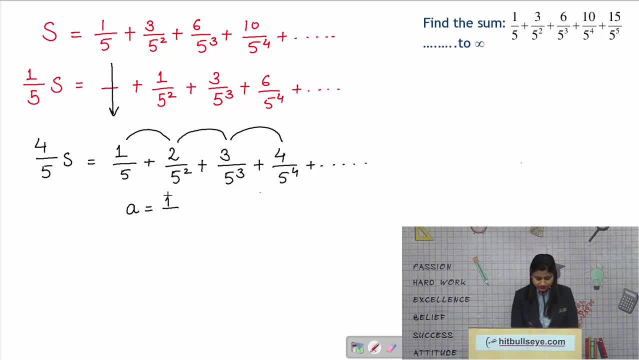 first term of AP which is 1 by 5 square and then we will take the subtraction which is 1 what is a common difference that is 1 again what is B B means first term of the GP it is 1 by 5 and what is a common ratio that is 1 by 5 again so 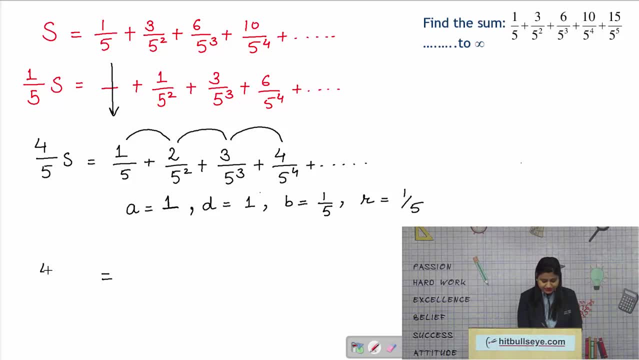 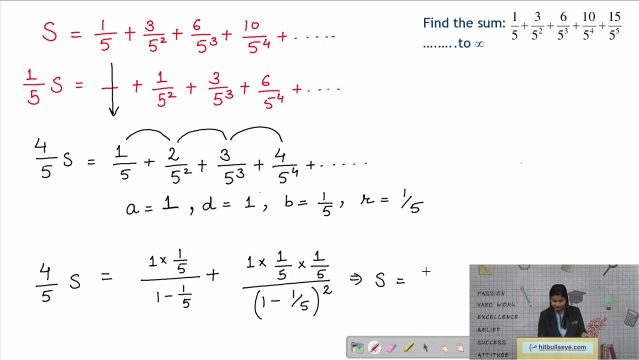 we will apply the formula here which comes out to be a B upon 1 minus R and plus D B R upon 1 minus R its whole square so if you solve it you will get the answer again I'm leaving the calculation part it comes out to be 25 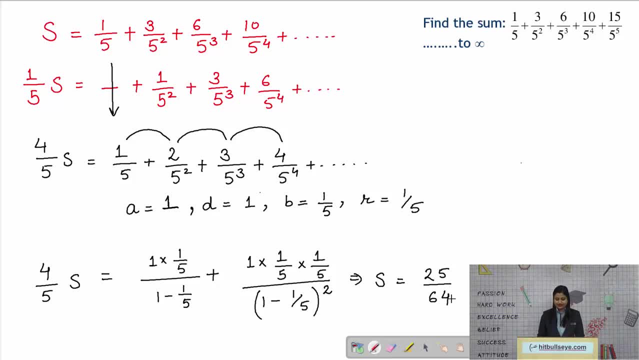 by 64 and that is the final answer in this case now let us move to next 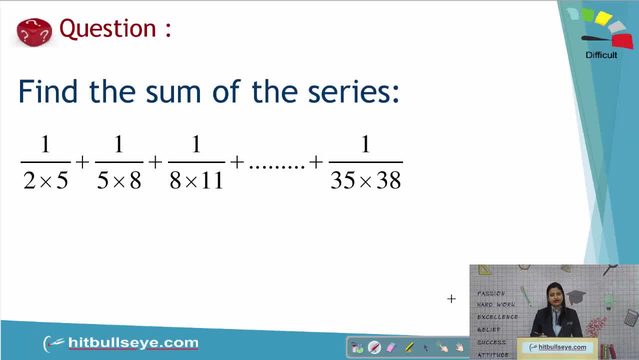 question again a new kind of series we want to find the sum of the series 1 upon 2 into 5 plus 1 upon 5 into 8 plus 1 upon 8 into 11 plus so up to plus 1 upon 35 into 38 there is a pattern going on if you observe what does the difference every time this is 3 1 upon 2 into 5 2 plus 3 will become 5 5 plus 3 becomes will become 8 and so on. So how to solve these kind of sums? Again there is a method. In this 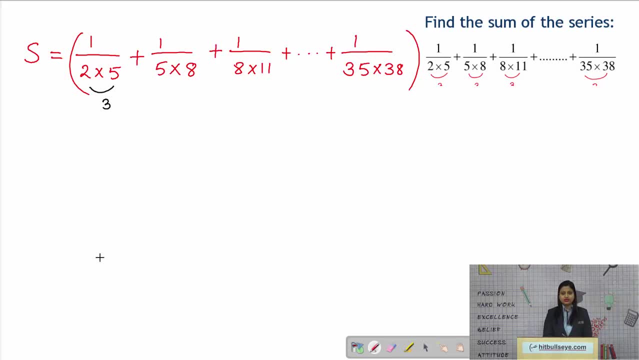 case you will take the difference. As you can see this is 3. So we will multiply and divide the whole series by 3. I mean it will become 1 by 3. We are dividing it by 3 and we are multiplying it 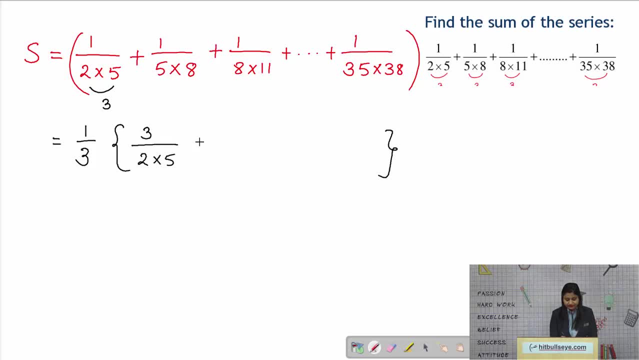 by 3. So it will become 3 upon 2 into 5 plus 3 upon 5 into 8 plus so on up to 3 upon 35 into 38. What is the usage of this? See now this 3 can be written as 5 minus 2. 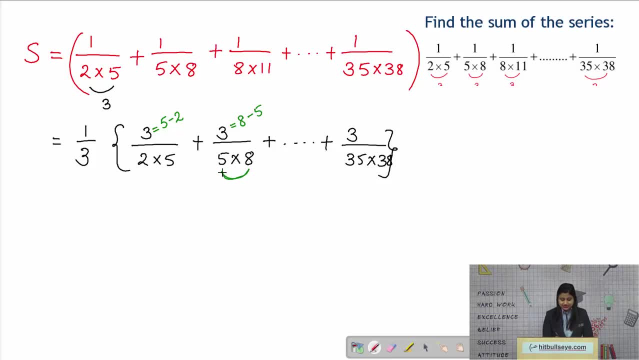 It can be written as 8 minus 5. As you can see here we have 5 into 8. That's why I have written this as 8 minus 5. Since we have a 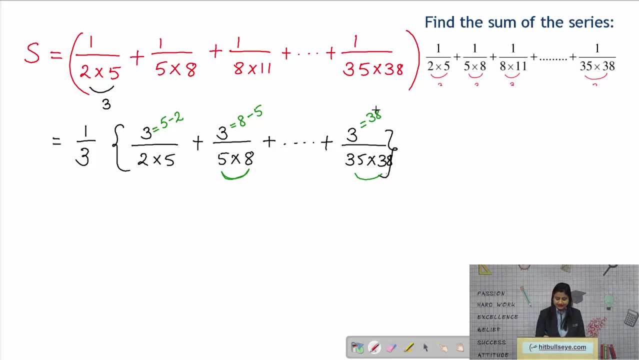 denominator 38 into 35 that's why we are writing it as 38 minus 35. So if we take the very first term it will become 5 minus 2 upon 2 into 5. If we separate them it will become this. 5 upon 2 into 5 minus 2 upon 2 into 5. Similarly the next term will be 8 upon 5 into 8 minus 5 upon 5 into 8. 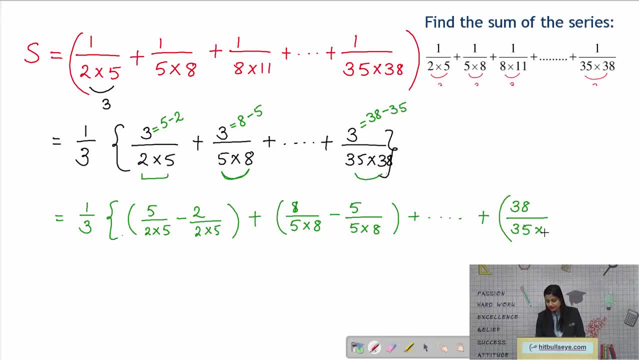 The last term will become 38 upon 35 into 38 minus 35 upon 35 into 38. Now see the magic. What is the usage of all these things? 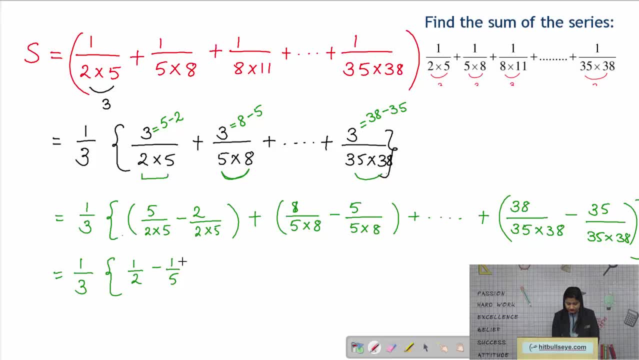 become 1 upon 2 minus 1 upon 5. They got cancelled. Plus 1 upon 5 minus 1 upon 8. Plus 1 upon 8 minus 1 upon 11. The last term will become 1 upon 35 minus 1 upon 38. Now, if we take the second term of first bracket and the first term of second bracket, they got cancelled. 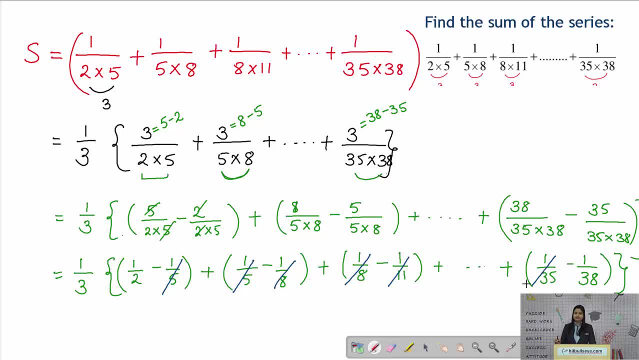 So, all the term will get cancelled except the first and the last term and this will happen always. So, my answer will become 1 by 3 half minus 1 upon 38. If we solve it, we will get 3 by 90. That will be the final answer in this case. So, directly we can learn, we can assume that whenever the last term is mentioned, we will take only the first 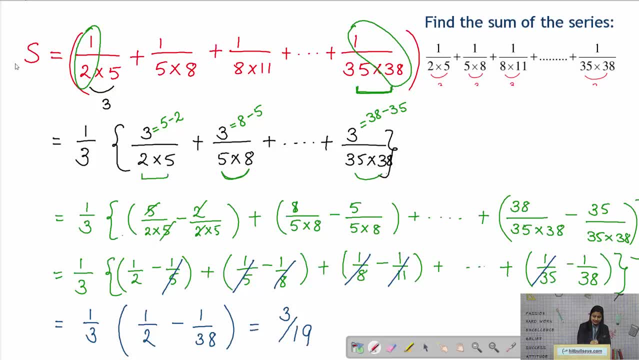 term and the last term. So, my answer will become half minus 1 upon 38 into 1 upon the difference. What is the difference here? 3 will be the difference here. So, that will be the final answer in this case. 3 by 90, this is the answer. 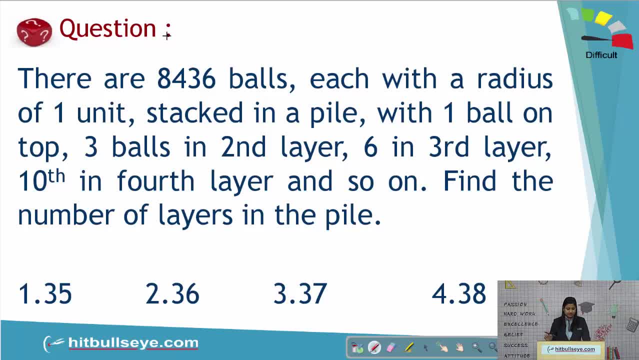 Now, let us move further. A huge question. It says, there are 8, 4, 3, 6 balls, each with a radius of 1 unit, stacked in a pile with 1 ball on top, 3 balls in second layer, 6 in third layer, 10th in fourth layer and so on. Find the number of layers in the pile. 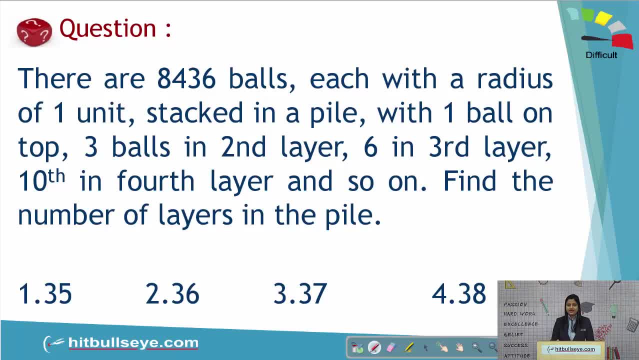 So, let us understand the meaning of this question. We have some balls in a pile. We have 1 in the first pile. We have 1 in the second pile. We have 1 in the third pile. We have 1 in the fourth pile. We have 1 in the fifth pile. We have 1 in the sixth pile. Then 3 in the second layer. Then 6 in the third layer. And 10 in the fourth layer. And we do not know the number of layers here. That is the question. So, let us say there are n layers. So, I am writing this as n terms. And this total comes out to be 8, 4, 3, 6. 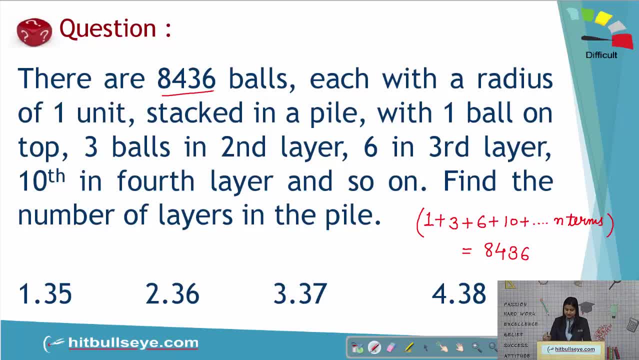 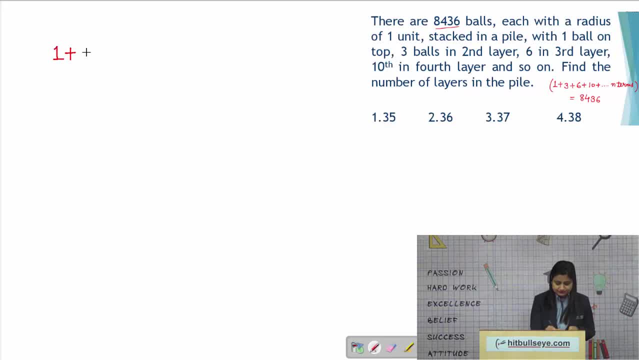 We want to calculate n here. So, let us see. We will take the help of C. We will take the series again. It says 1, 3, 6, 10, sewn up to n terms. This is not a direct AP, GP or AGP series. But we can observe that the difference here is 2, 3, 4 and sewn up to. How can we solve these kind of series? We will try to write the nth term of these kind of series. So, we will try to write the nth term of these kind of series. As we can see that T1 is 1 here. I mean the first term. T2 is 3 here. That is 1 plus 2. We are adding 2 to first term. Then we have T3. That is 1 plus 2 plus 3. Then we have T4, which is 1 plus 2 plus 3 plus 4. So, by generalizing, we can say that Tn will be nothing but summation n. See, the first term, we are taking only 1. The second term, we are taking 1 plus 2. And in the third term, we are taking sum of all natural numbers up to 3. In the fourth term, we are taking sum of natural numbers up to 4. So, we can generalize that in tn, we will take sum of first n natural numbers. So, it will become sigma n. We have a formula for this. 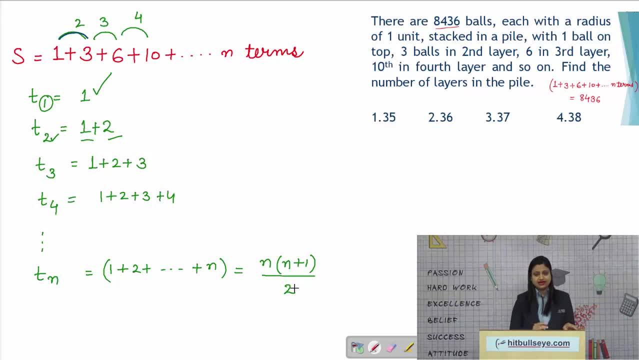 This is n into n plus 1 by 2. That is our nth term. Now, we want to write sn here, sum of n terms. So, how can we do this? Nth term can be written as half into n square plus n. 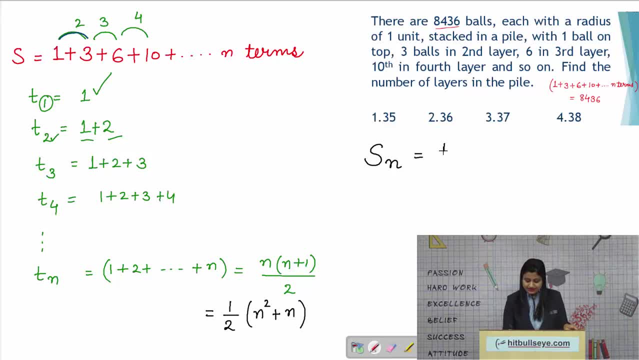 So, if we apply sigma here, it will become half sigma n square plus sigma n. How? 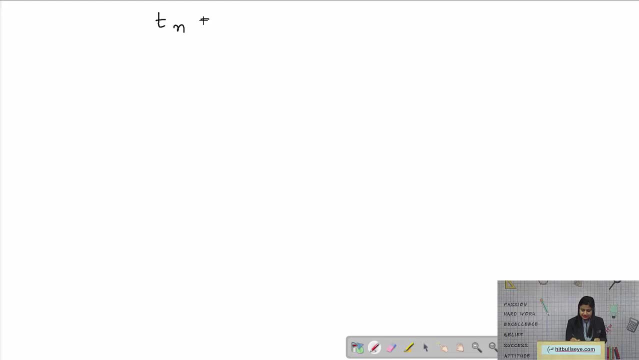 How come? Let us see. See, our tn is half n square plus n. What will be t1? If we write in this manner, it will be 1 square plus 1. What will be t2? It will be half of 2 square plus 2. And so on up to tn. It will be half of n square plus n. We want to calculate sn 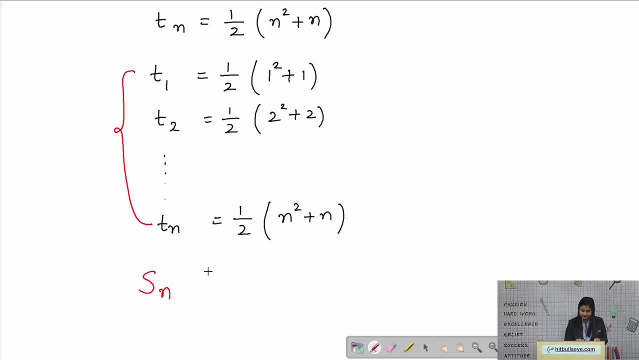 here. What do you mean by sn? That is sum of first n terms. So, if we combine them, we will get 1 square plus 2 square plus so on up to n square. That is the first column. 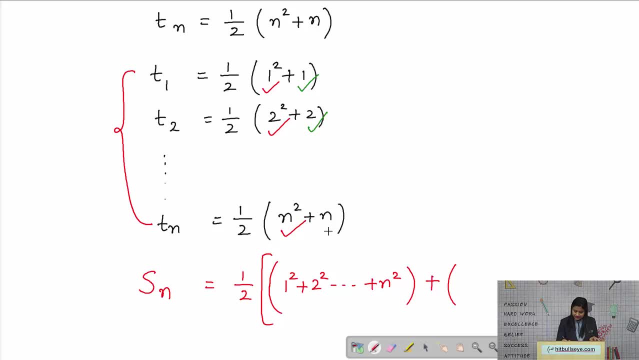 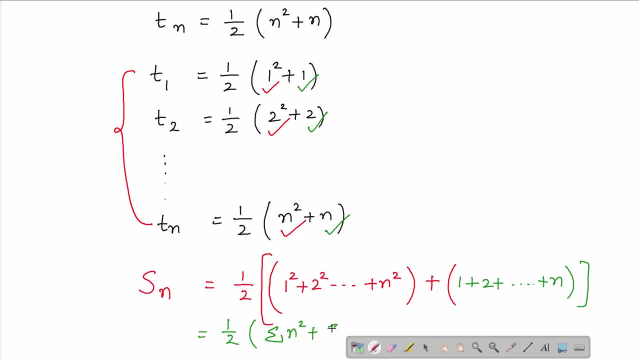 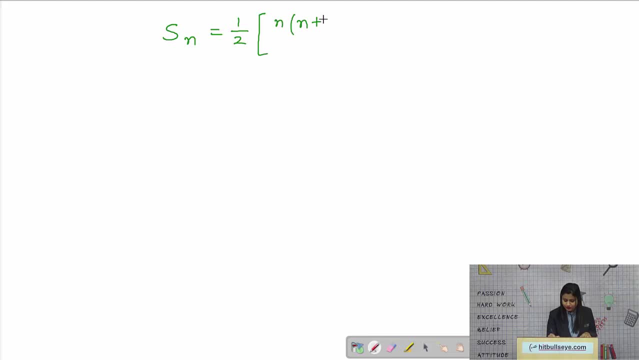 of sigma n square plus sigma n. Let us solve this. What is sigma n square formula? It is n into n plus 1 into 2n plus 1 divided by 6. Plus, what is sigma n formula? n into n plus 1 divided by 2. So, first of all, we will take n into n plus 1 divided by 2. Common. We will be left with 2n plus 1 divided by 3 plus 1, which will become n into n plus 1 divided by 4 into 2n plus 4 divided by 3. If we solve it, the final expression will become n into n plus 1 into n plus 2 because 2 will be common here, divided by 6. Now, this sum of n terms, if we add n to n plus 1, we will get n into n plus 1 divided by 3. So, this 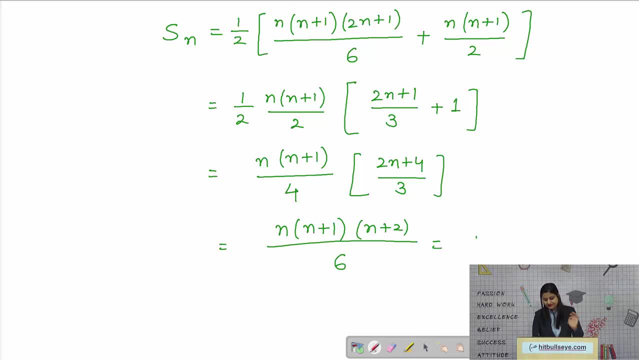 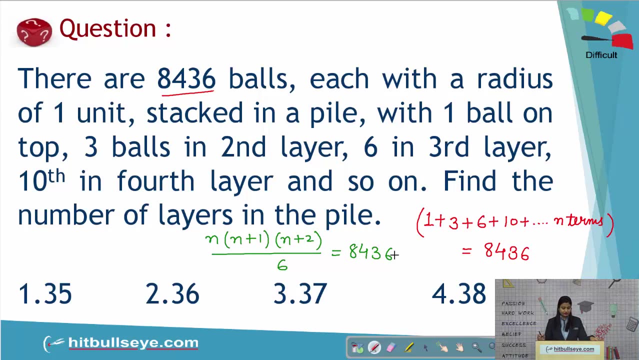 will become n into n plus 2. We will get n into n into 5. Isn't that simple? Entonces, ya que Lotsa gente está pensando que este no será la misma覺as considerando que tendremos n elementos, este se da como 8, 4, 3, 6, para que si solucionamos se tomará la respuesta. Vamos por las opciones. Leviabasde la opcion 2,élé isso es la opción 2. Así que habrá 36 elementos en ese panel. 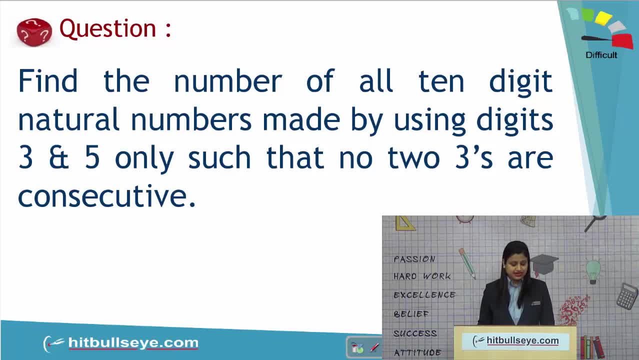 Finalmente, este es un crookedo trabajo. La siguienteругa serie de Fibonacci dice... Former funcional de Fibonacci dice... Find the number of all ten digits natural number de todos los doces natural identificadosx by using digits 3 and 4. ¿Y el número de todos los doces naturales creados por usando the three and four digits? We are giving n to n into n of've movie value and we are maintaining the number! 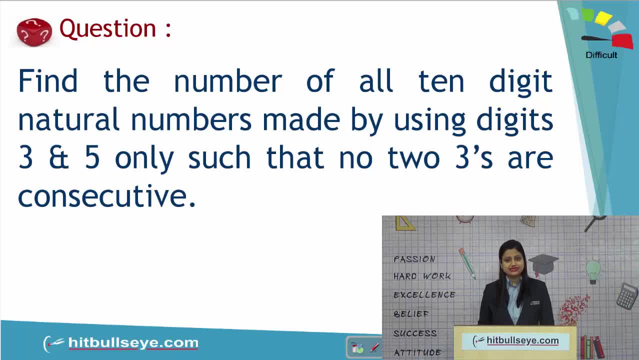 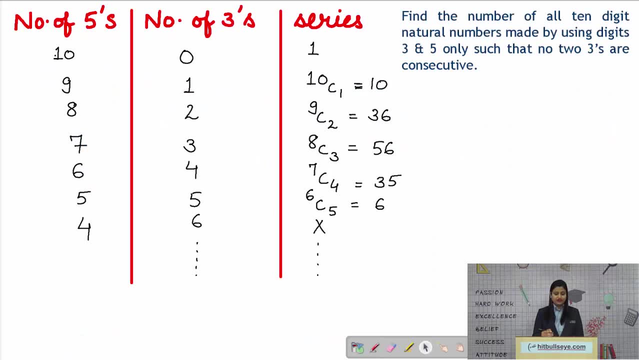 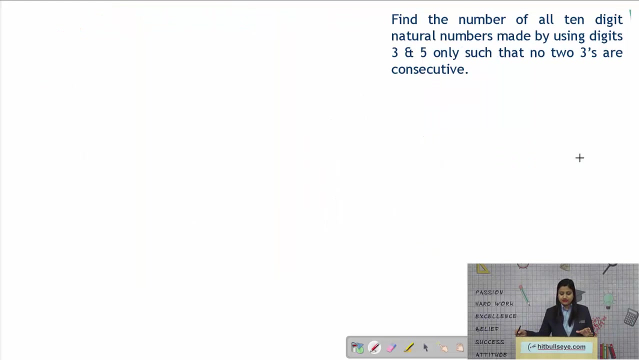 only such that no two threes are consecutive. No two threes are together. So, what is our conventional approach? We will try to make cases since it says that no two threes are together consecutive. So, we can take number of 5s and there will be no 3. How many such numbers are possible? There is only one number that is all 5s. Then we will take the second case where number of 5s are 9 and there is only one 3. So, 3 can occupy any of the 10 places. That's why there are 10 numbers possible. If we keep on going in such manner, we will have many cases and by adding all of them, we will get 144 as the answer. But it is cumbersome. So, we will make use of a beautiful series which is known as Fibonacci series. See, we will go by taking smaller length of the number. Let us take there is only one digit number. So, I am applying the same condition that we want to make numbers by using only 3 and 5 and no two threes are consecutive. So, 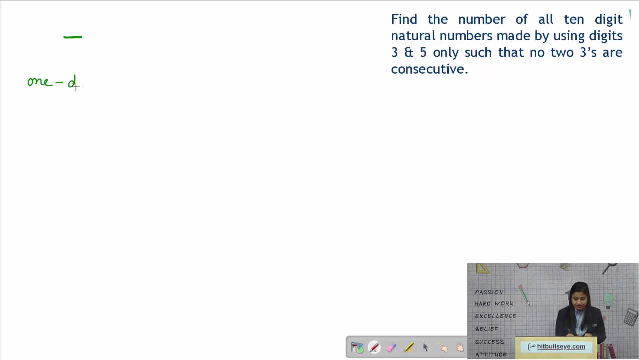 we are talking about one digit number. So, how many numbers are possible? 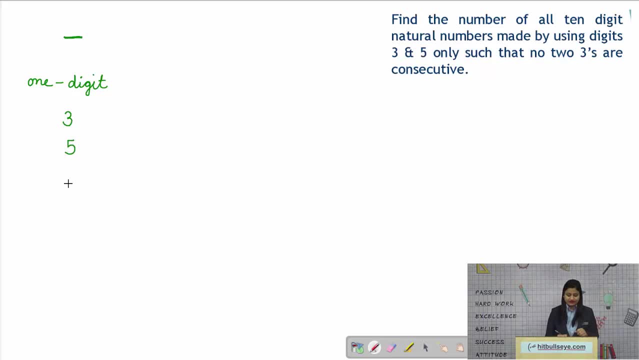 Only two. Either it will be 3 or it will be 5. So, in total, how many numbers are possible? 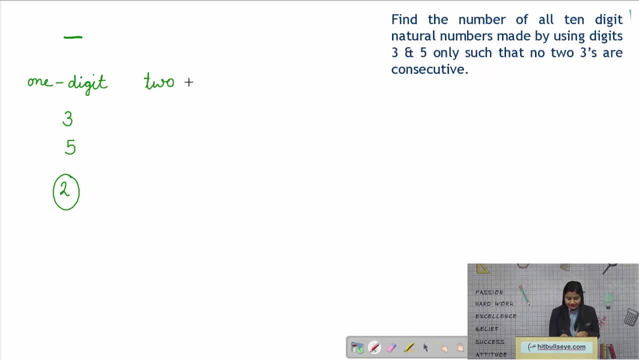 Two. What about if I take two digit numbers? So, if we make cases, since our condition is no 2, threes are consecutive, number can be 55, it can be 53, it can be 35, but it cannot be 33 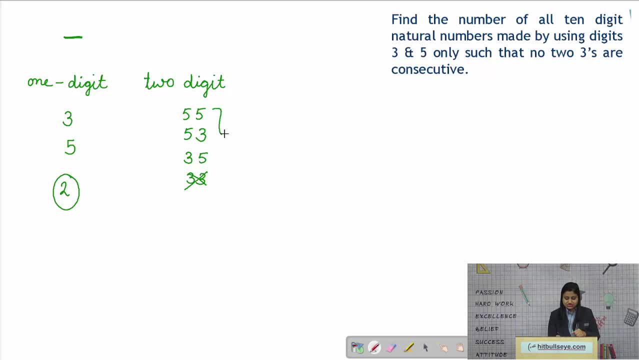 because of the condition given. So, how many such numbers are possible? They are three in total. 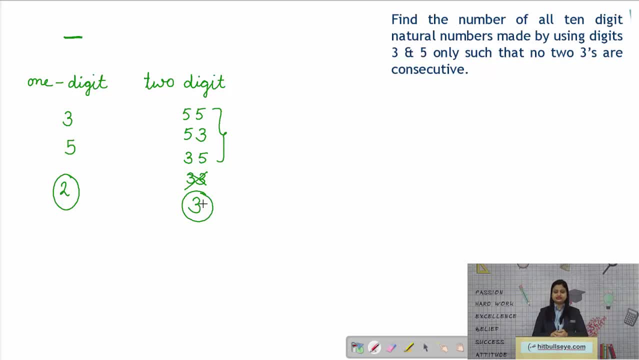 So, we have seen, if we are talking about one digit such number, they are two in number. 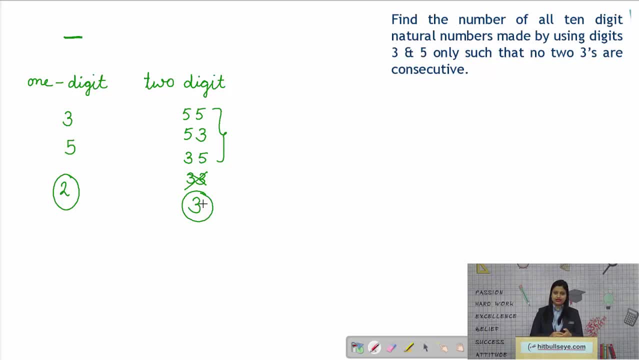 If we are talking about two digit numbers, they are three in total. What about if we take three 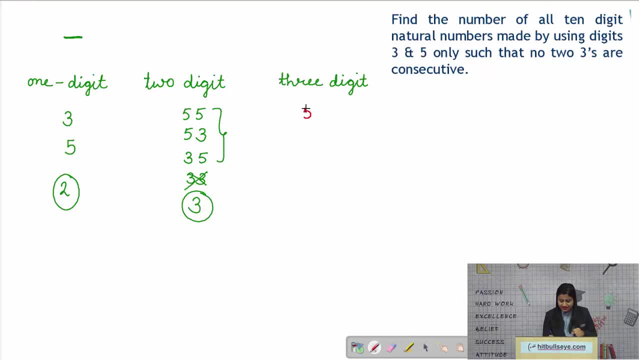 digit numbers? Either my number will start with a 5 or my number will start with a 3 and there are two places remaining. So, if we take the first case in which the number is starting with 5, remaining two places are nothing but all the two digit numbers which are satisfying the same condition and we have calculated that there are three such numbers. Once again, if we are starting our number by 5, either my number will be 55, 555 or it will be 555. So, if we are talking about two digit numbers, we have to take the first case, which is 553 or it will be 535. So, these are nothing but the case which we have calculated previously. Now, let us come to the second case where my number is starting with a 3. After 3, you cannot take a 3 because of that condition that 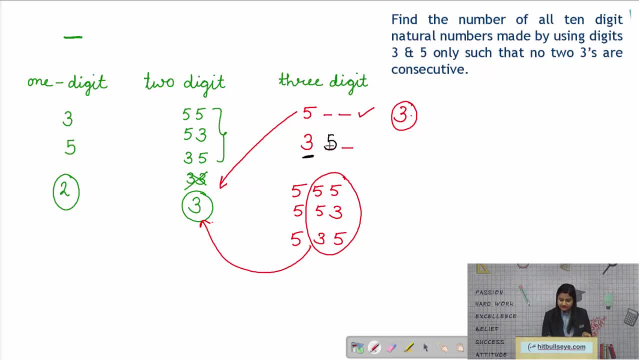 no two threes are consecutive. So, we have to take a 5 on the second case. So, the remaining numbers are nothing but all the one digit numbers which are satisfying the same condition and we have 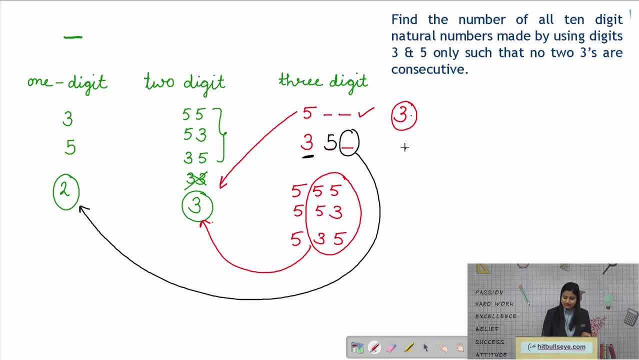 calculated it previously. So, how many such three digit numbers are possible? They are five in 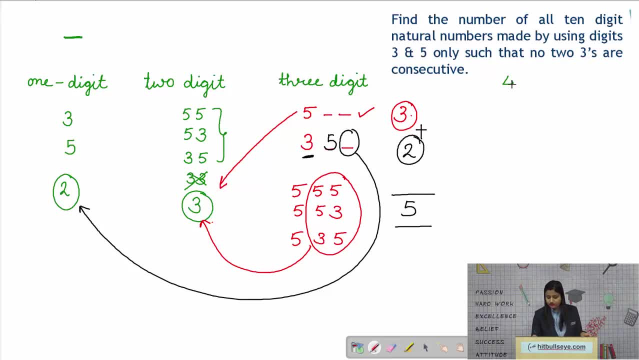 total. Once again, if we talk about four digit numbers, either my number will start with a 5 or my number will start with a 3. Since we are talking about four digit numbers, three places are 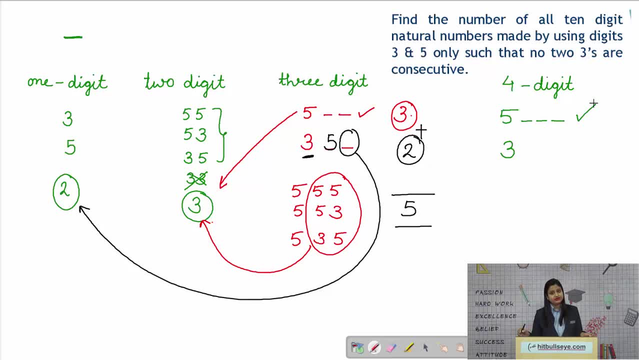 remaining. So, if we take the very first case where the number is starting with a 5, we still have three digit numbers. So, if we take the first case where the number is starting with a 5, we still have three places to fill. So, these three places are nothing but all the three digit 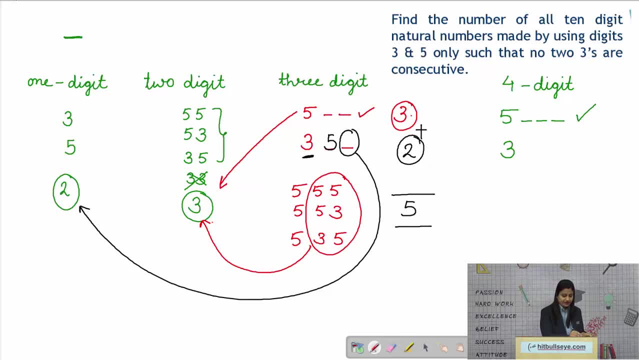 numbers which are satisfying the same conditions and we have calculated those in the previous case. 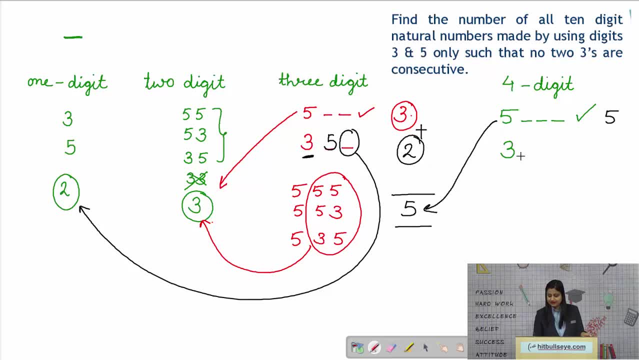 They are five in total. Similarly, if we take the next case where our number is starting with a 3, 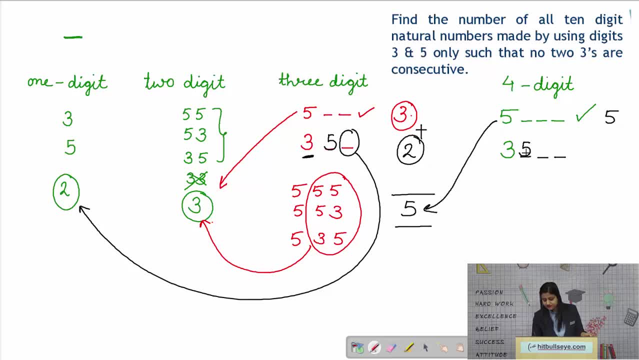 after 3, you cannot take a 3. That is why we will put a 5 here. So, we are talking about all the two digit numbers which are satisfying the same condition. So, if we take the next case where the number is starting with a 5, we still have three places to fill. So, these three places are the same condition that we have calculated previously. So, it will be nothing but in total 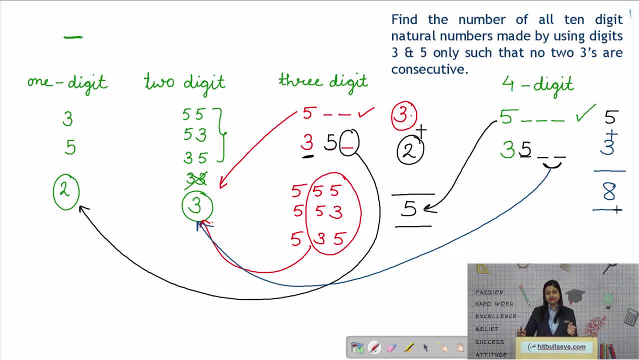 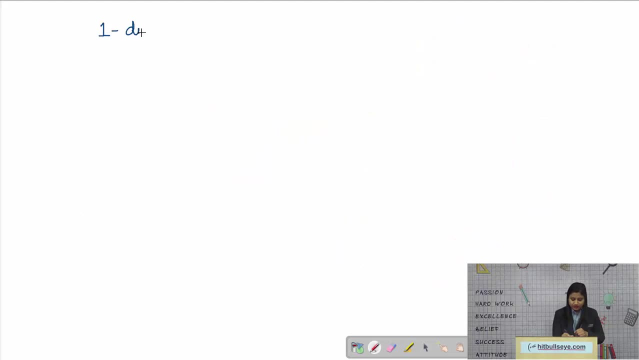 8. So, every time we are calculating, we are increasing the length of the number. Suppose we are calculating five digit numbers. It will be nothing but sum of previous two places. So, we can say that if we talk about one digit number, they were 2. We can say that if we talk about one digit number, they were 2. So, we can say that if we talk about one digit number, they were 2. So, we talk about two digit number, they were 3. Three digit, that is nothing but the total of previous two terms, that is 5. Four digit, again the sum of previous two terms, that is 8, 3 plus 5. If we go on in this manner, we can calculate 10 digit number which comes out to be 144 and 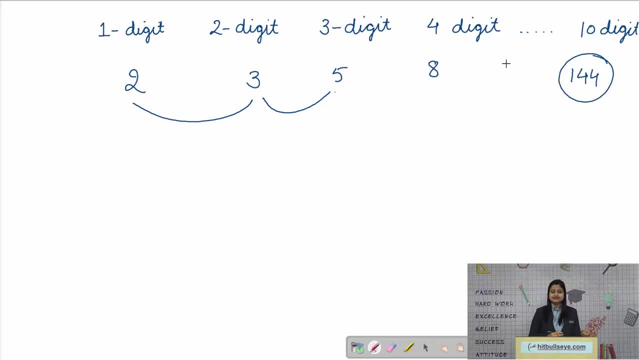 that was the answer in this question. So, this kind of number is going to be 144. So, we are going to write it here as an8 and that is going to be 4, so 4 is larger than the number of times which is from the answer out. So, we can write this answer in three digits. So, we have cease 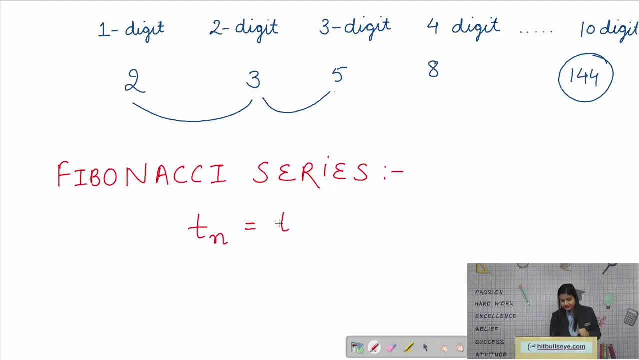 mode in here where the term is the same like sweep mode and in this we can just write the number of times which is from the answer which comes out to be 4 and then let me give it a little bit, it can easily be District number which will be 4 which is from the answer out. So, when mengles sometimes every time it will be 3. How many are there in this function? 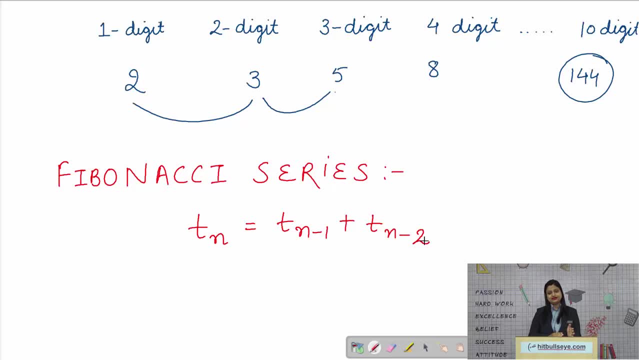 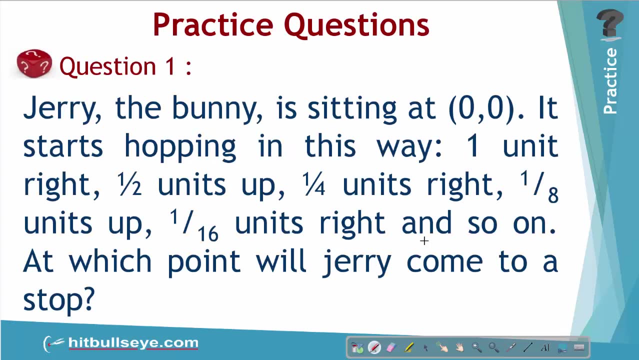 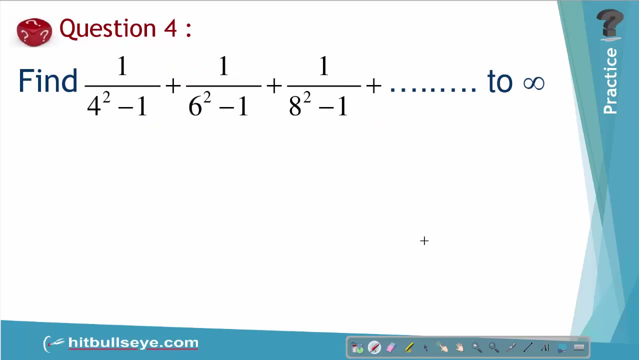 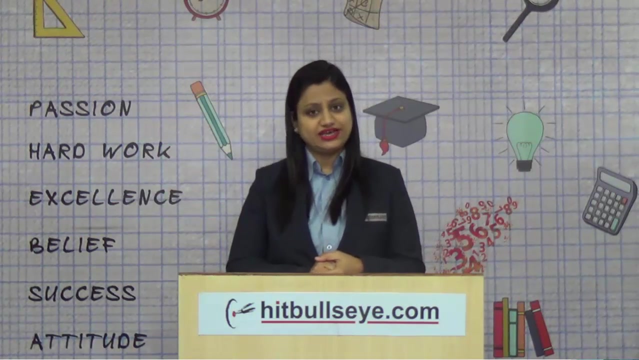 in a jiffy because we have to calculate a series only, not so many cases. So, answer is 144 in this case. Now, these are some practice questions and these are the answers. For more videos and more concepts, log on to hitbullseye.com. Thank you so much. Happy learning. you